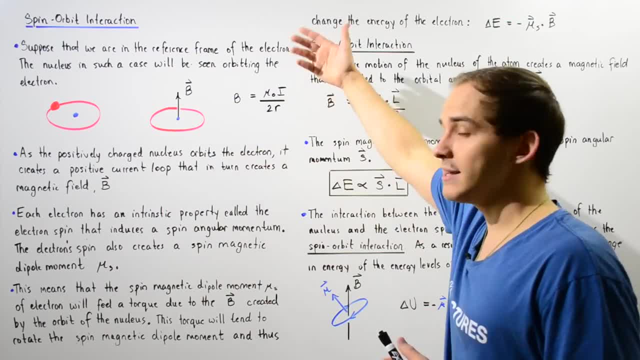 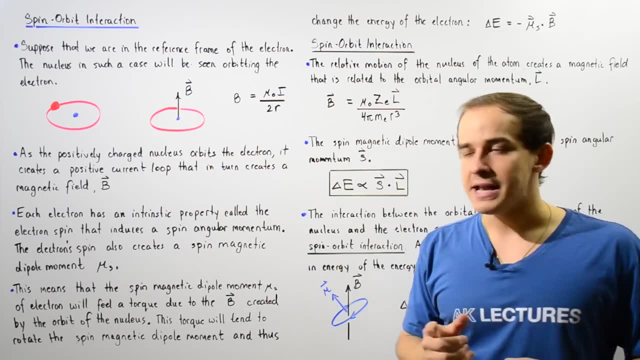 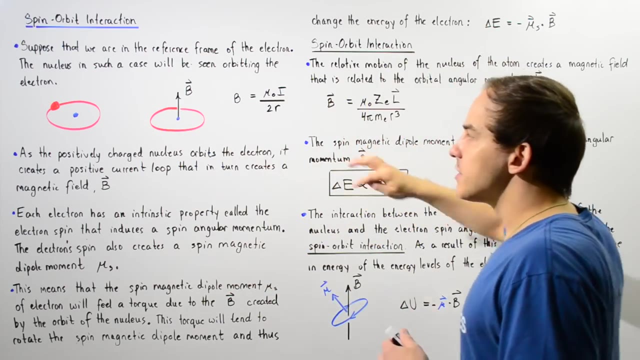 of it is given by this equation: where mu naught is a constant, I is the quantity of electric current and R is the radius of the circuit. The magnetic field B is given by the right hand rule and in this case the magnetic field B points upward, as shown in the following diagram. 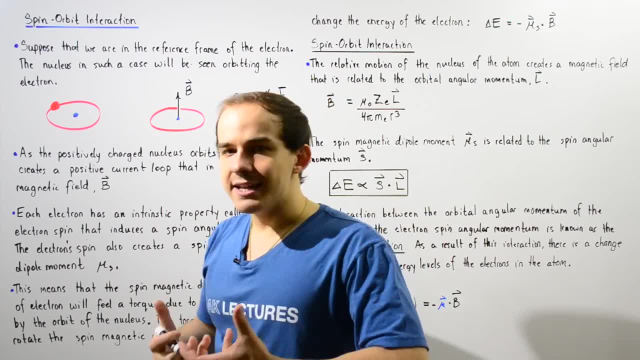 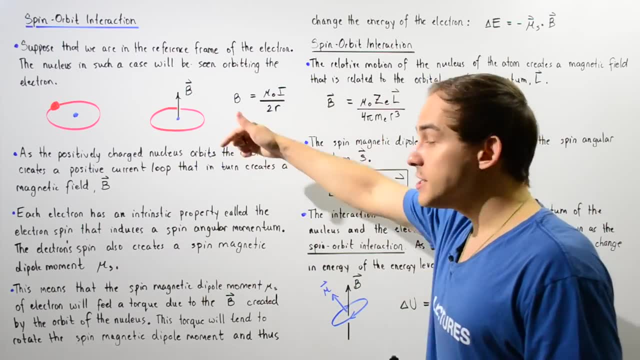 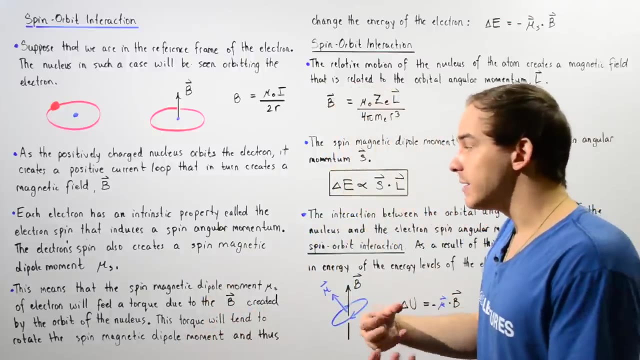 Now recall that any electron has an intrinsic property known as the electron spin, and the electron spin creates the spin angular momentum of that electron. So the electron has an angular momentum of a plug. So the electron has an angular momentum, momentum that is created by the electron spin. Now the electron spin also induces. 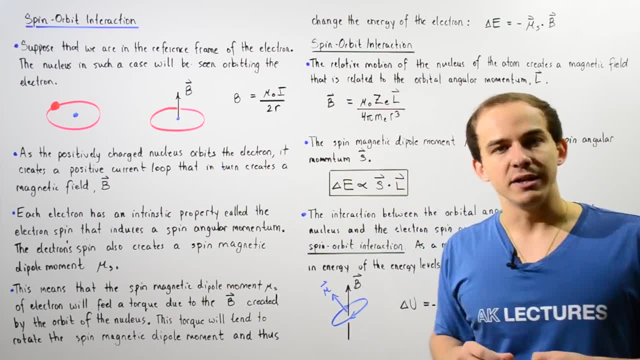 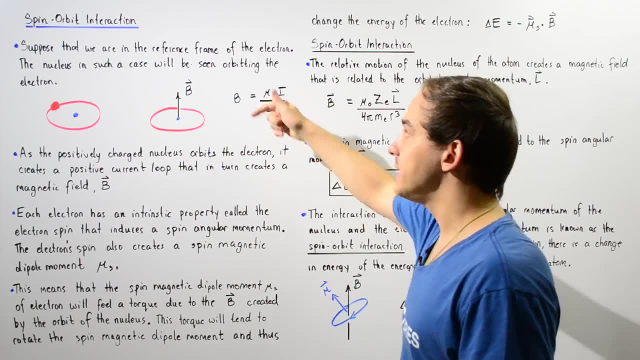 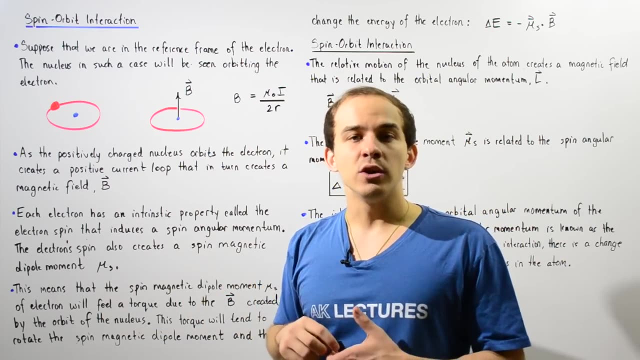 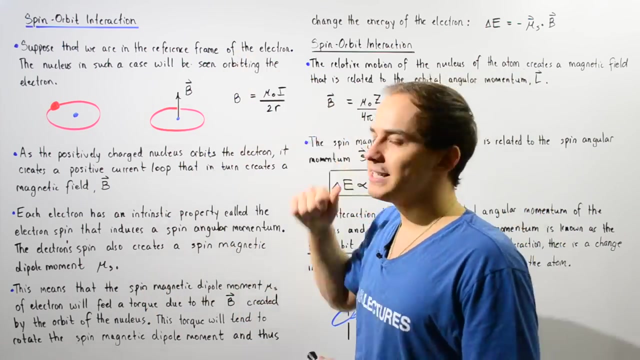 or creates a spin magnetic dipole moment given by mu s. and basically, whenever we place a magnetic dipole moment into a magnetic field, what will happen is the magnetic field B will create a torque that will act on the magnetic dipole moment, mu, to orient it along the same direction as the magnetic field lines. 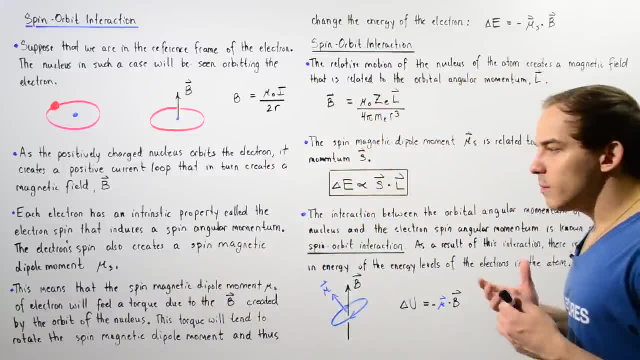 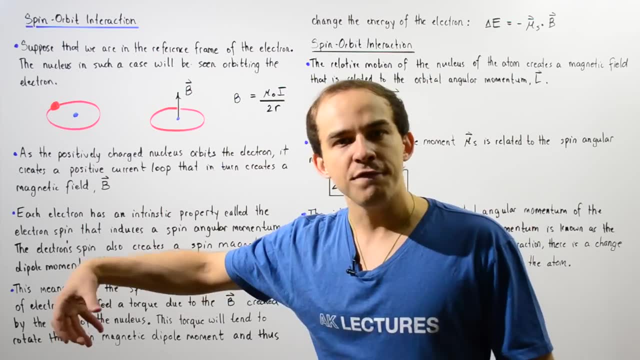 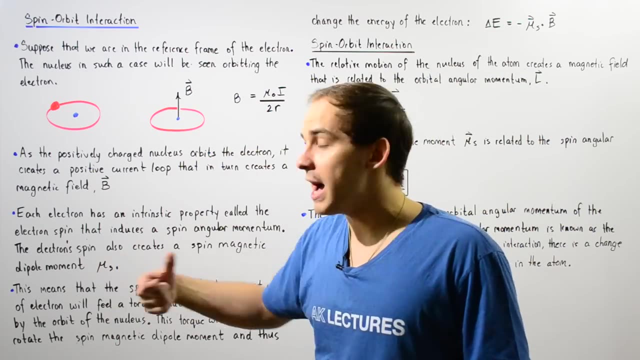 created by the magnetic field B. So basically, this means that the spin magnetic dipole moment mu s of the electron will feel a torque as a result of the magnetic field B created by the orbit of the nucleus, created by the relative motion between the electron and the proton in the nucleus. Now this 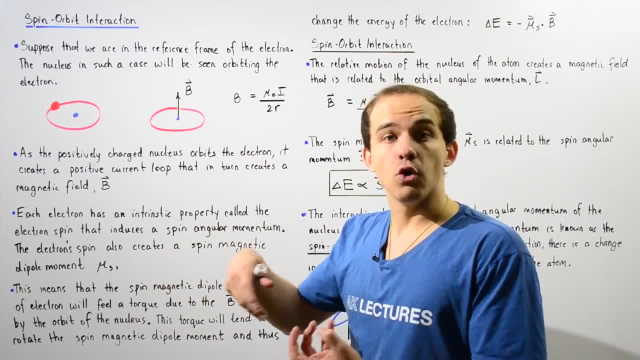 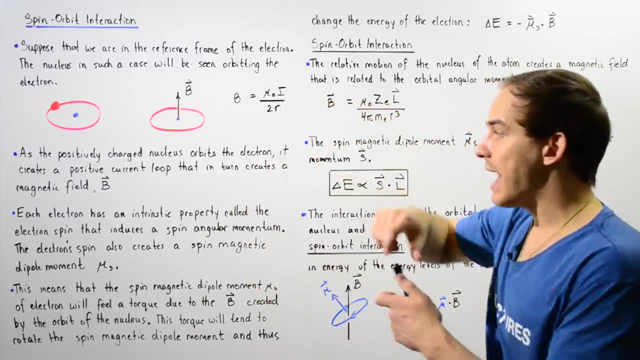 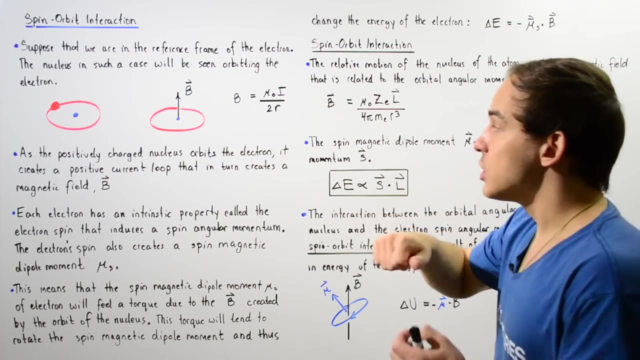 is a very important point because if you have a magnetic dipole moment, mu, that is, this torque will basically tend to orient or rotate that spin magnetic dipole moment along the same direction, along the same axis as the magnetic field lines of that magnetic field B. and that means that as the torque acts on the 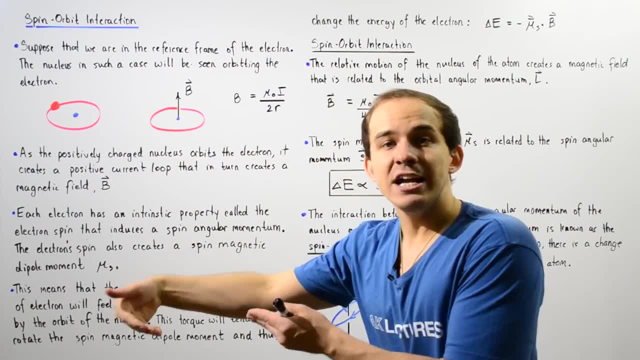 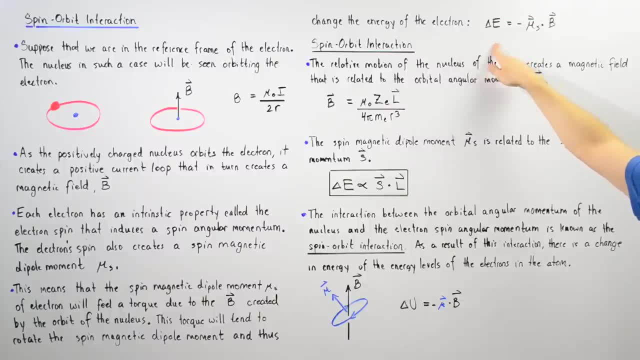 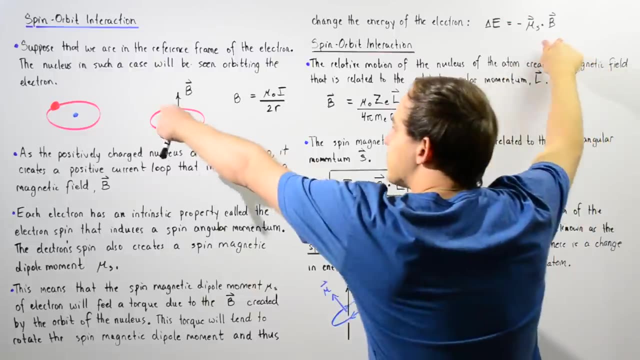 electrons magnetic dipole moment, it will change the energy of that electron by the following amount. So delta E, the change in energy is equal to negative- of the dot, product of the magnetic field vector created by the relative motion between the electron and our nucleus, as well as the mu s, where 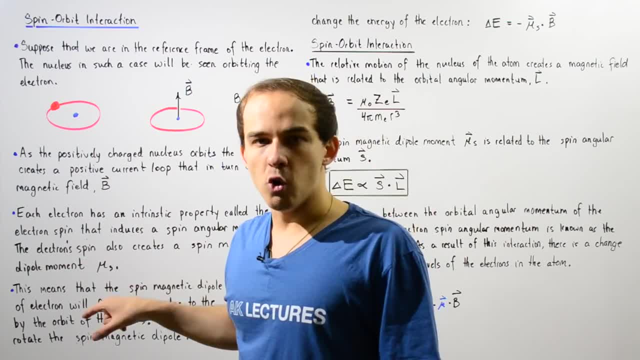 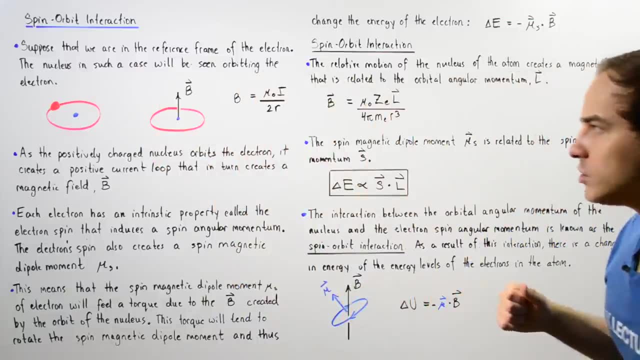 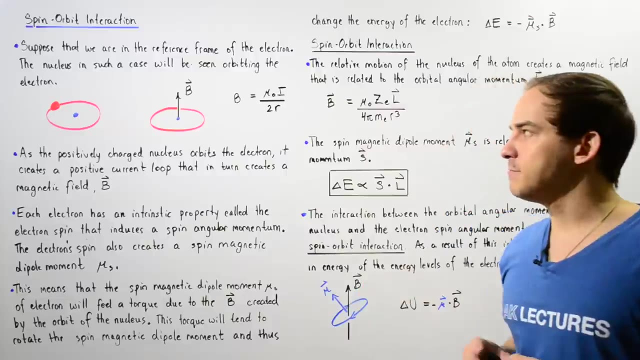 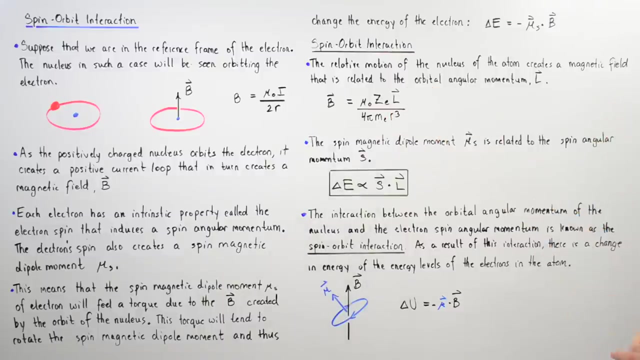 mu s is the spin magnetic dipole moment. Now the question is: what exactly is this spin orbit interaction? Well, to describe what the spin orbit interaction is, let's recall the relationship between the magnetic field B and the orbital angular momentum of our atom, So the relative motion. 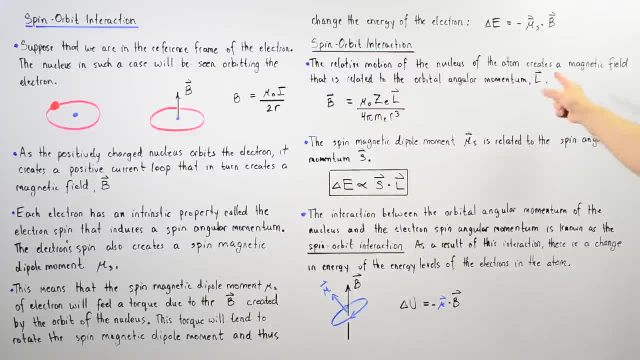 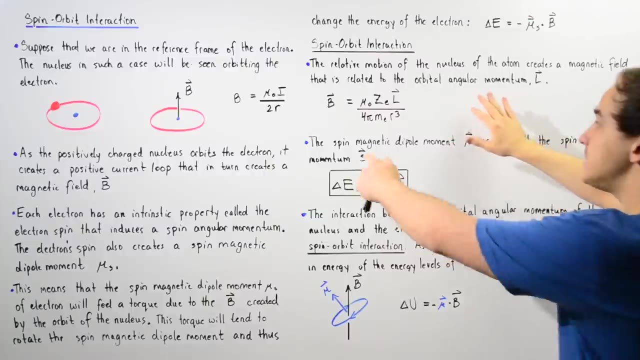 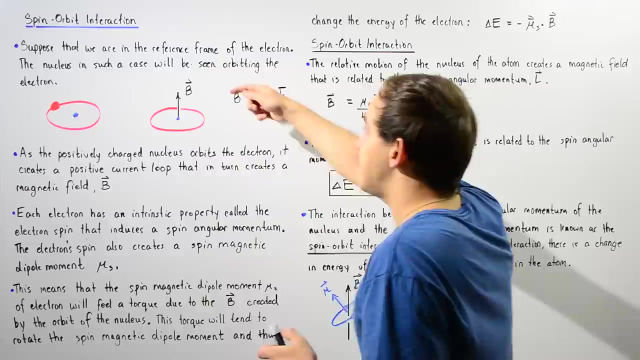 of the nucleus of the atom and the electron creates a magnetic field B, as we discussed just a moment ago. and this magnetic field B is related to the orbital angular momentum given by capital L and the relationship is given by this equation. So basically we can think, or another way we can think of this magnetic field B is in terms of the 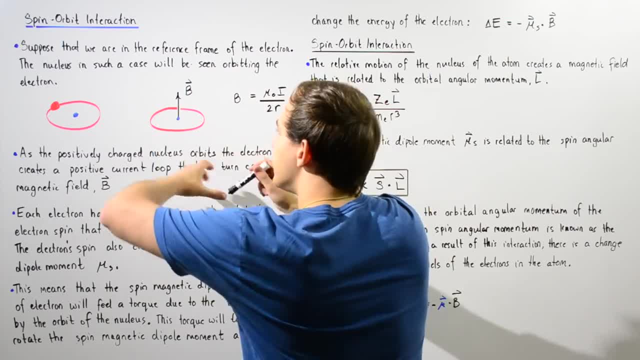 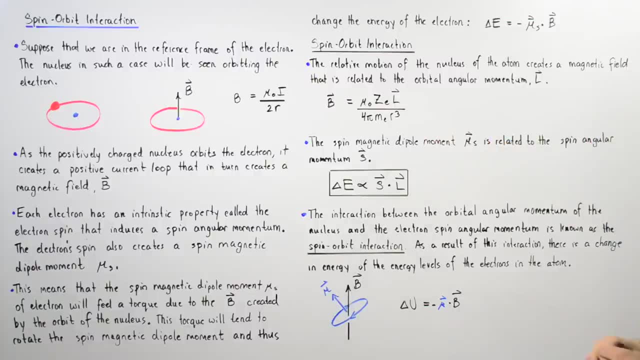 orbital angular momentum created by that nucleus's motion around our electron, and it's given by this equation. Now, another important relationship that we must remember is the relationship between the magnetic dipole moment, or the spin magnetic dipole moment mu s and our spin dipole moment. 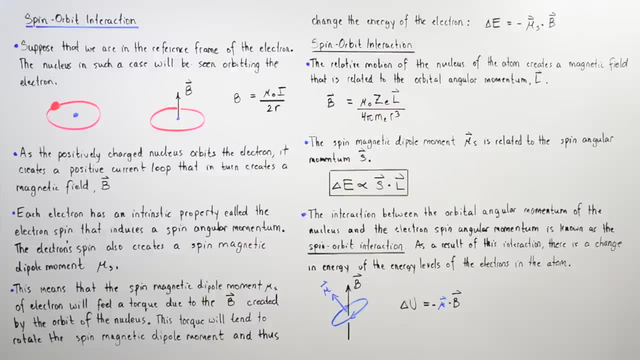 angular momentum. So basically, the spin magnetic dipole moment mu s is related to or is proportional to the spin angular momentum given by capital S, And that means another proportion that we can write is as following: So another way we can rewrite this equation is in the following format: 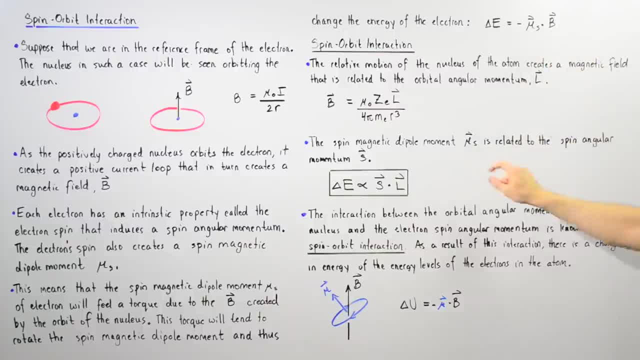 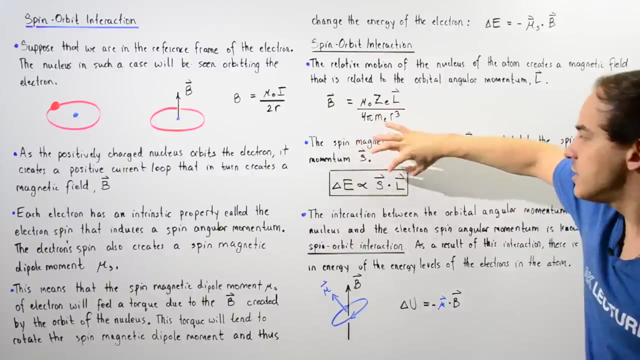 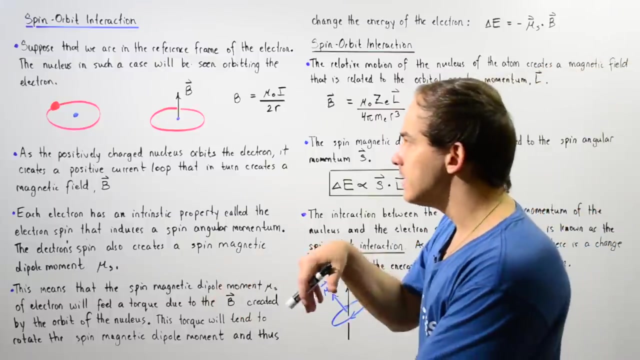 Because B is related to L and because mu s is related to S. if we take the dot product of these two vectors, so our orbital angular momentum L and the spin angular momentum S, we see that this dot product is directly proportional to the change in energy that our electron feels. 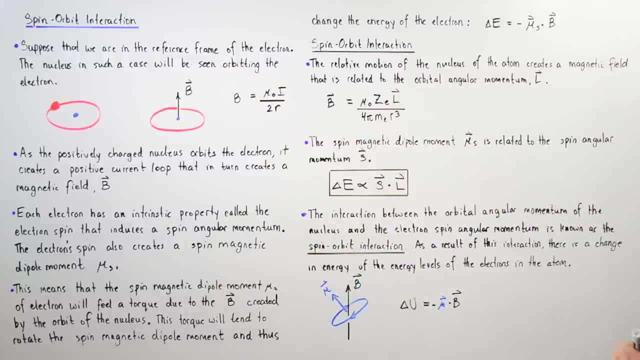 as a result of this magnetic field B. Now, the interaction between the orbital angular momentum L of the nucleus and the electron spin angular momentum given by S is known as the spin orbit interaction. And from this discussion we see that as a result of this, 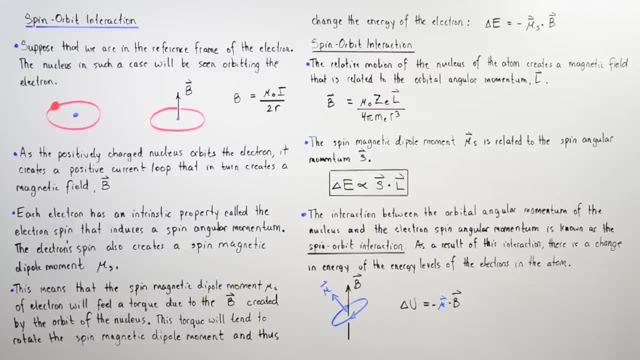 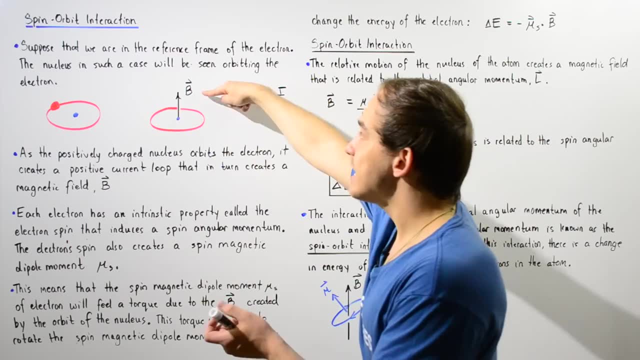 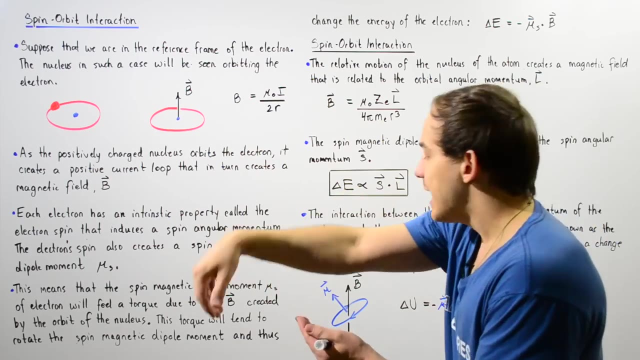 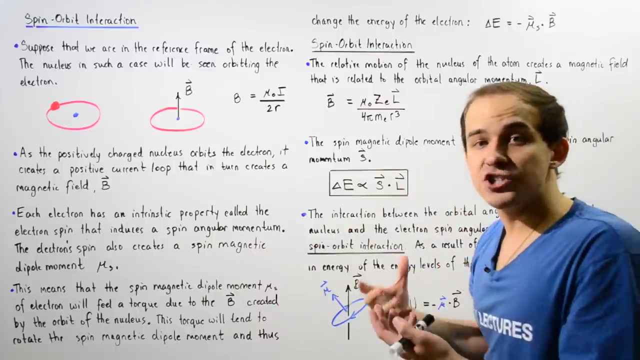 interaction there is a change in energy, of the energy levels of the electrons within the atom. because when that magnetic field B creates a torque that acts on the spin magnet dipole moment mu, it will basically rotate and as it rotates that electron that will change the energy. as per this equation, or 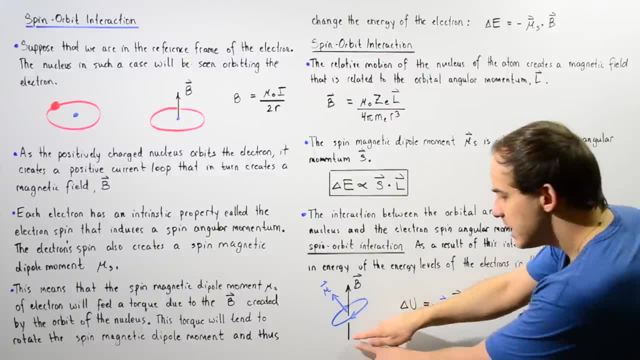 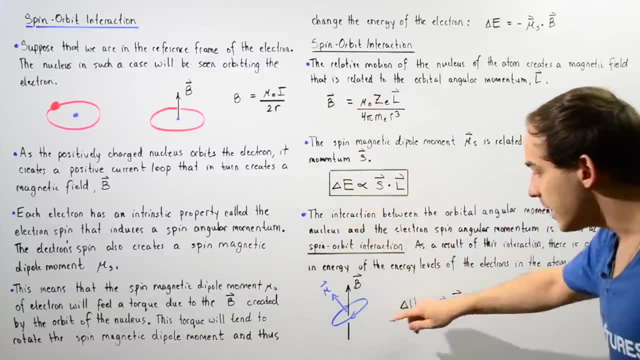 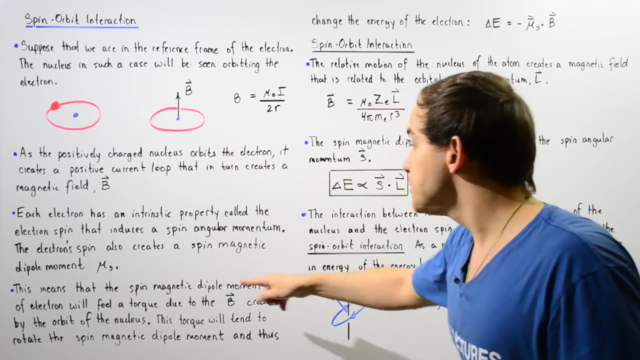 this equation. So basically let's imagine that the magnetic field B is given by this arrow, So the magnetic field B points upward and the electron basically spins around that nucleus and it creates the spin magnetic dipole moment mu s. So this is: 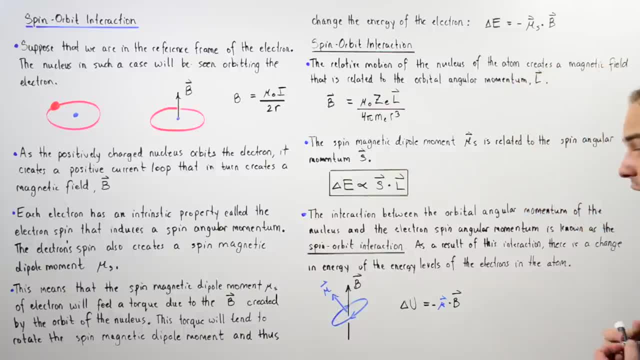 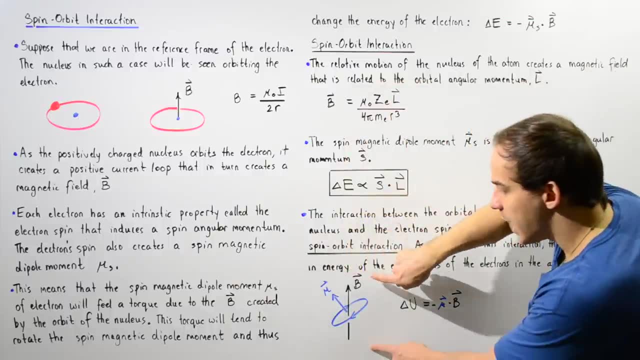 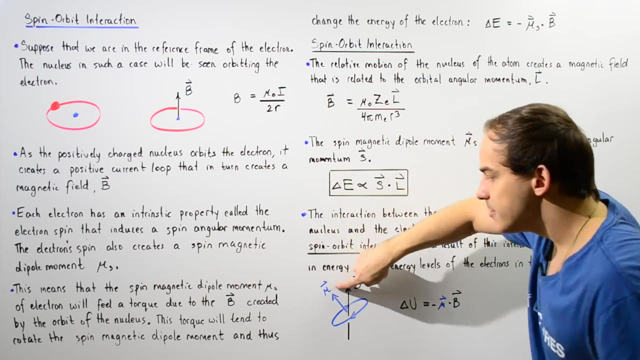 the spin, the magnetic dipole moment mu s, that is created as a result of the intrinsic electron spin of that electron and as we turn on this magnetic field B, the magnetic field B will create a torque that will tend to rotate this mu along the same axis as the direction of the magnetic field lines B. and when this 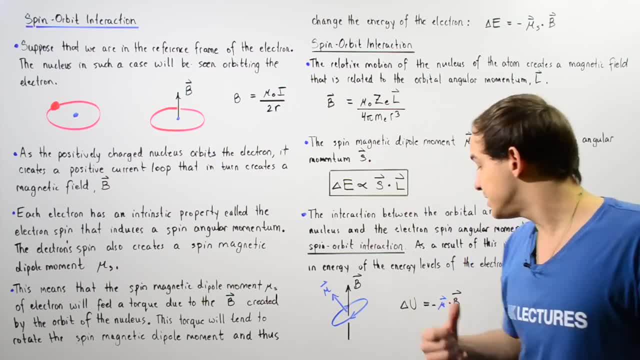 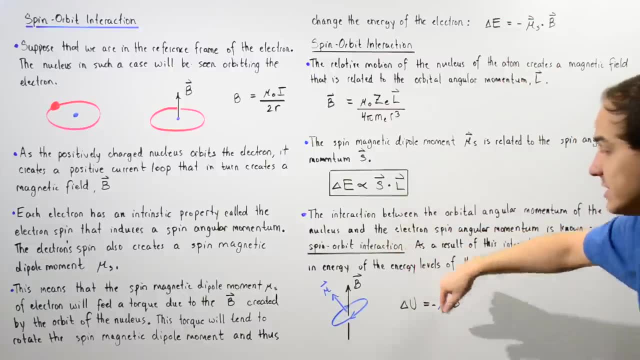 rotation takes place, the electron will change in its energy by this amount. So delta U is equal to negative mu, where mu is simply the magnetic dipole moment of that electron, as a result of the electron spin, and our B, where B is the magnetic field B that is created as a result of the relative motion between 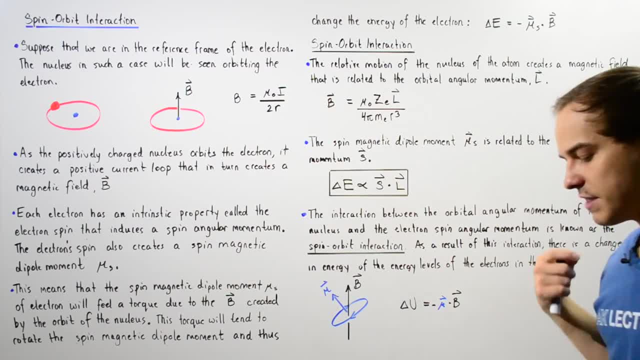 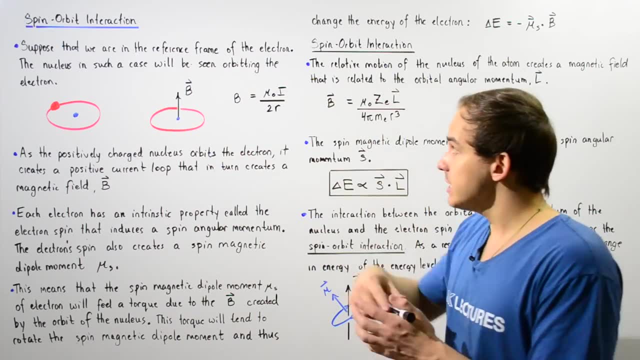 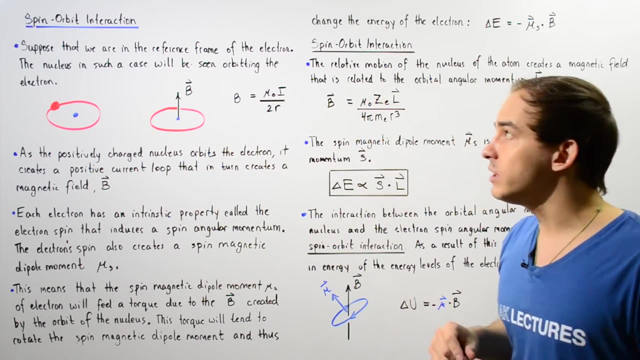 things, our electron and the nucleus of the atom. So basically the spin-orbit interaction is the interaction between the magnetic field B that is created by the relative motion between the electron and the nucleus, and the spin of that electron. So the spin magnetic dipole moment.